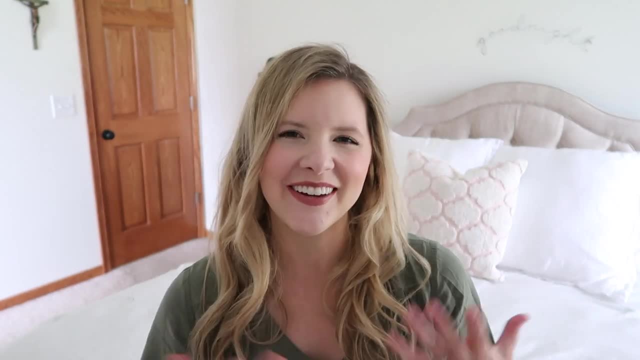 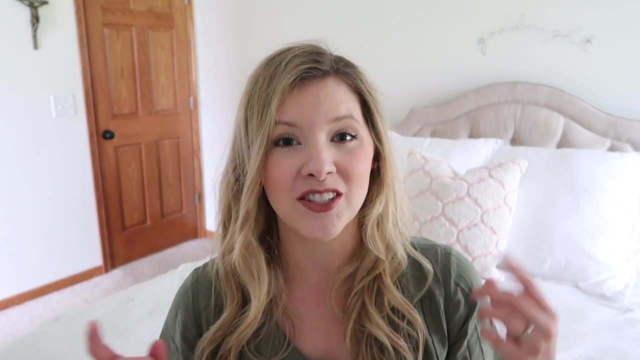 can make more pastel ones if you want, or more really vibrant ones if you want. So it's just kind of fun. So I will post written instructions below and I'll also post that over on my Instagram highlights. So if you want to just take a screenshot, I know I really like to do that when- 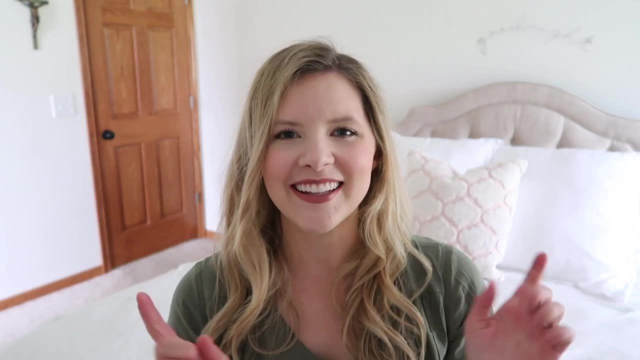 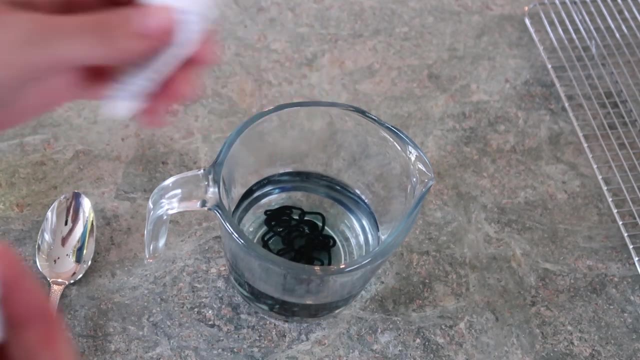 people post recipes and things. I just take a screenshot so that I have it on my phone. So, yeah, let's get right into the video and I'll show you how I make this play-doh. So first you're going to mix together your wet ingredients, So I'm just adding the food coloring to the water. 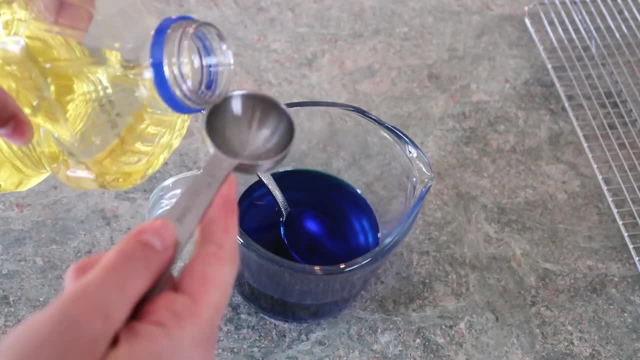 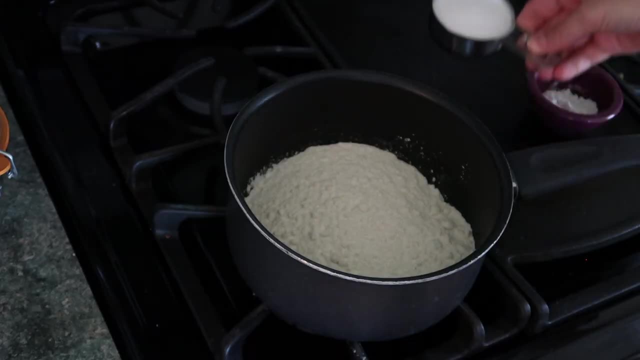 and I use gel food coloring, but you can really use whatever kind of food coloring you want- And then you're just going to add vegetable oil to that and stir it up. Then, in a saucepan over on your stove, mix together the flour, salt and cream of tartar. 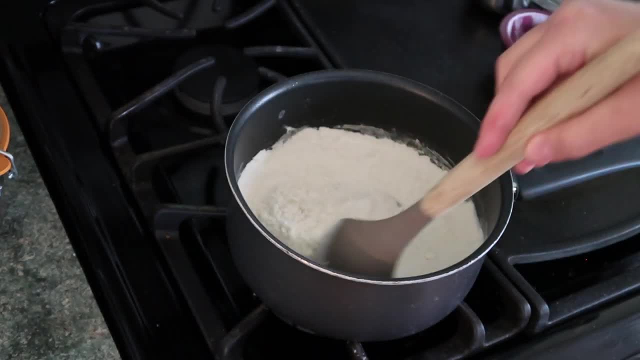 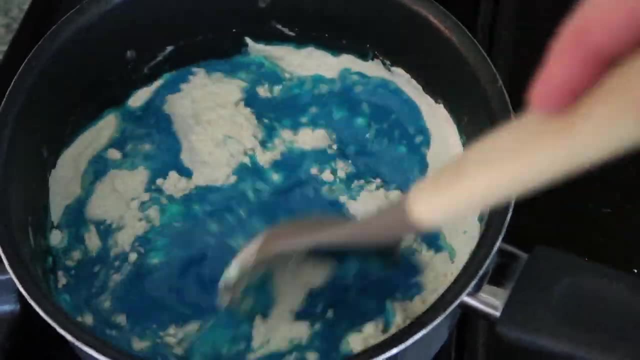 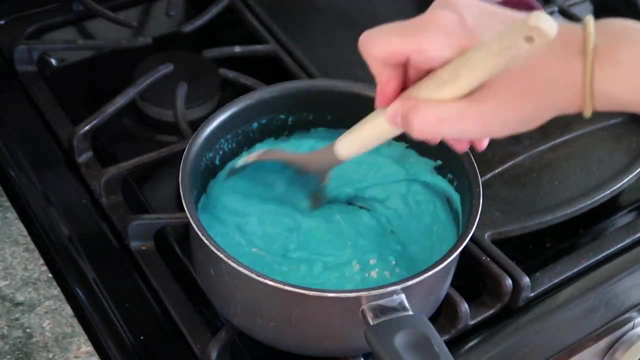 And then just add the water mixture to the flour mixture, Turn your stove on medium- maybe medium low- heat, And now you're just going to start stirring. And I sped this up, but you're just going to keep stirring, keep stirring And eventually, as you'll stir, 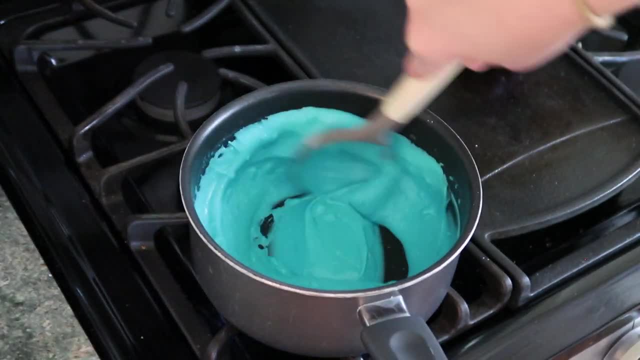 you'll notice that it'll start to get kind of lumpy, which is a good sign, And then it'll really start to get thicker. And that's how you know it's going to get thicker, You know it's becoming play-doh. 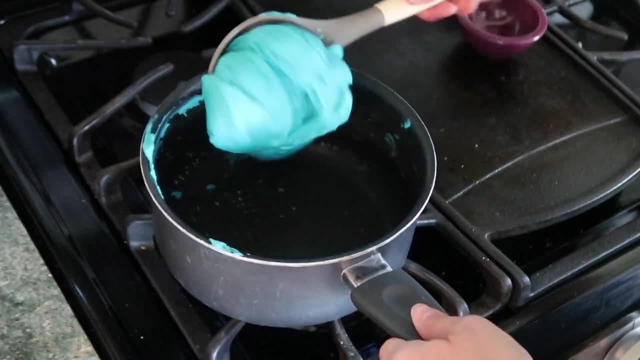 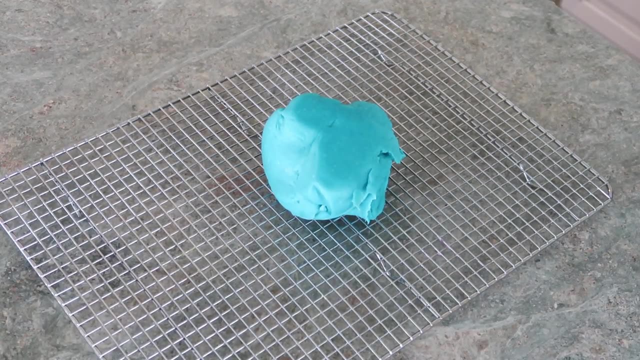 When it's all done, it comes together into one big ball like this and your play-doh is done. So next I just put it over on like a wire rack or just some kind of surface to cool down, And I did a little close-up here so that you can see how nice it looks. 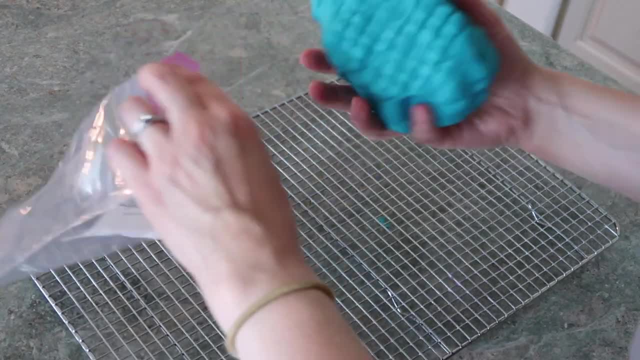 You can see how nice and squishy this play-doh is. So to store it, I just like to store mine in a Ziploc bag and just kind of squeeze all the air out, But you can store it in really any type of food storage container. 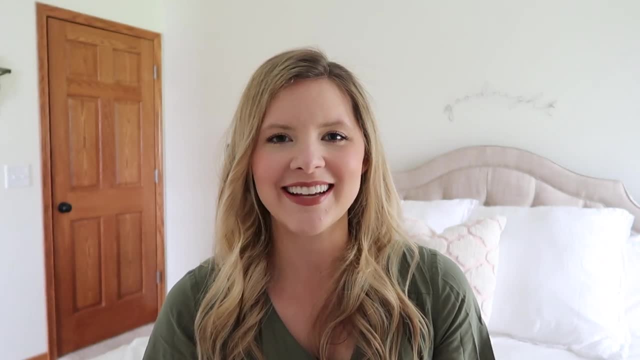 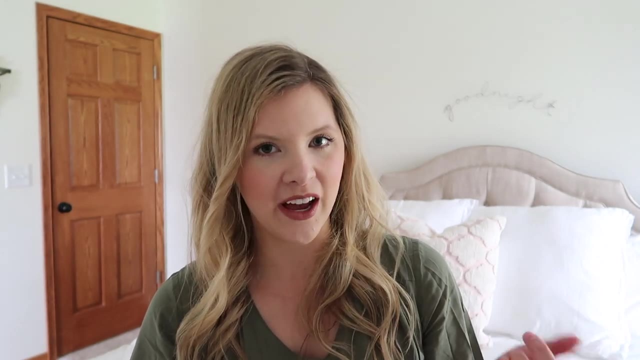 I hope you guys enjoyed this. Please let me know if you make it and be sure to tag me on Instagram so that I can see Be sure that you're subscribed to my channel and you can also click the bell notifications if you want to be notified every time I post. I'll see you guys in my next video. Bye. 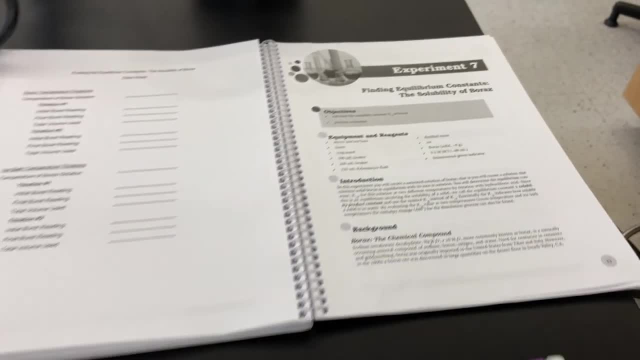 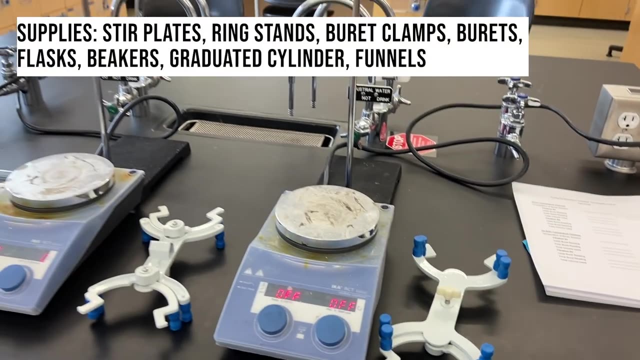 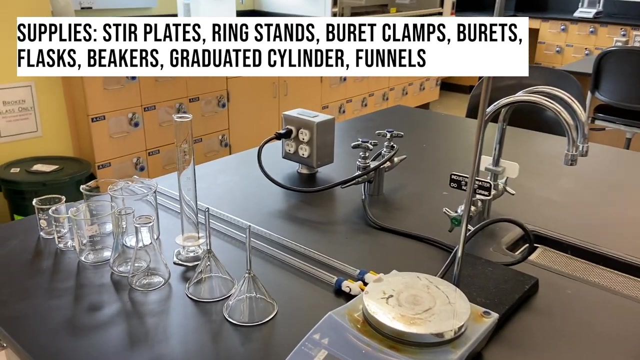 Today we will be exploring equilibrium constants through the solubility of borax. So to do that we will be doing a couple titrations. So we've got a setup of ring stands, stir plates, some burette clamps and, of course, some burettes and some other pretty.